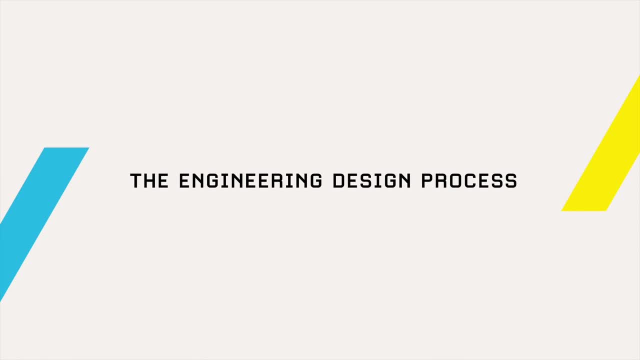 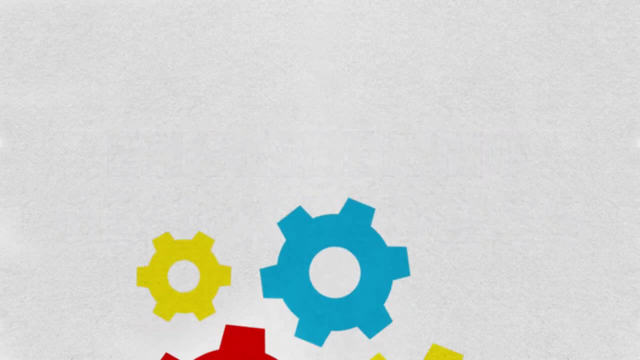 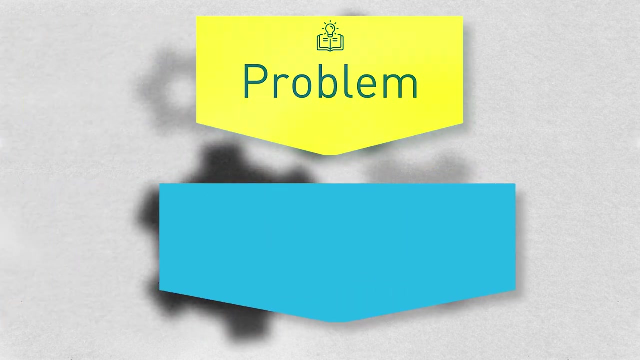 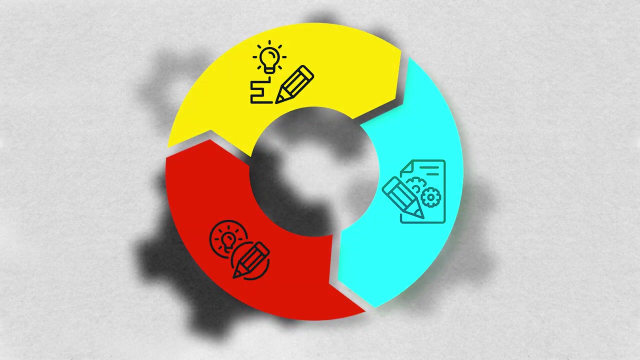 Engineers use the engineering design process to solve problems. You may be familiar with a scientific method or have used it to test hypotheses in science class. The engineering design process is similar. It's a series of steps we can use to solve a problem. It's useful because it's open-ended and allows for multiple solutions to the same problem. 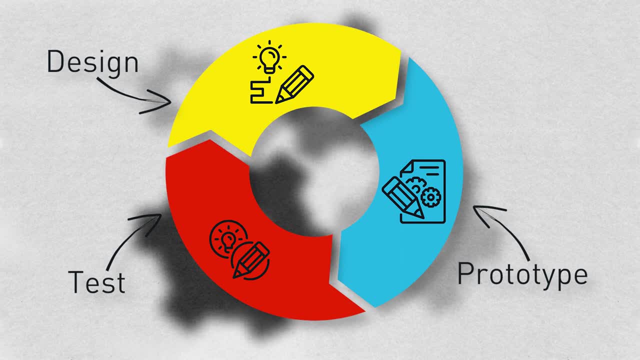 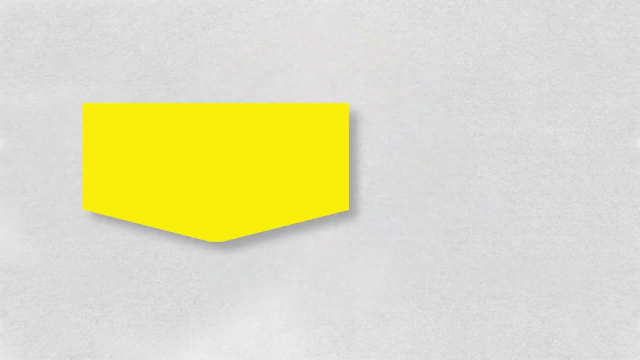 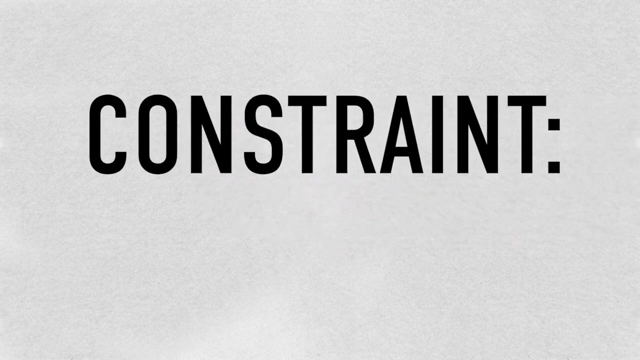 It's also iterative, which allows us to test new solutions and encourages us to try again when our solutions don't work the first time. First step: define the problem. What's the issue? This is also where we think about constraints. What are the limitations we have in solving the problem? Let's see how this works in real life. 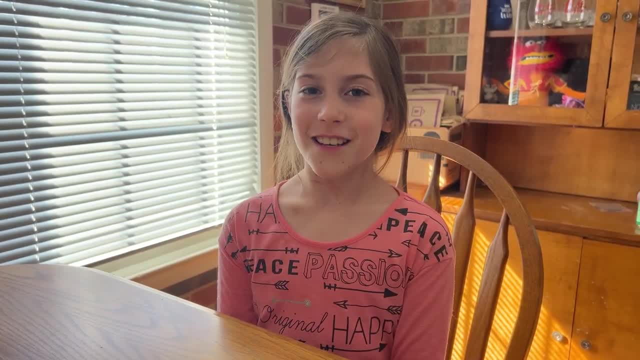 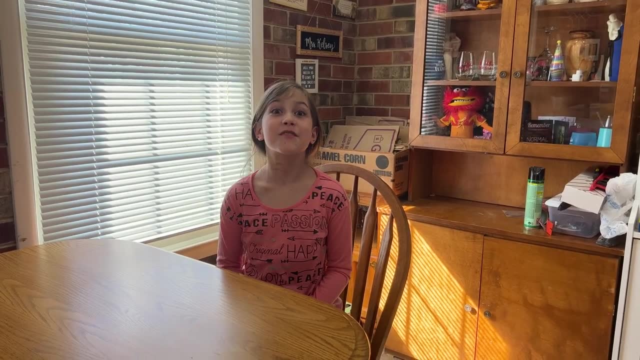 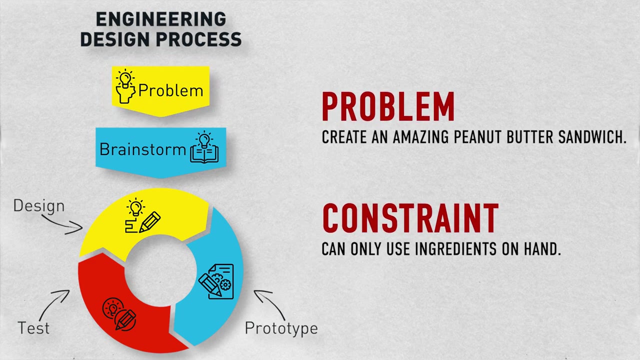 I'm starving. I want a peanut butter sandwich, but not just a plain peanut butter sandwich. I'm so hungry I need to start making this. Our friend needs to be able to make a better PB&J using ingredients they already have at home. 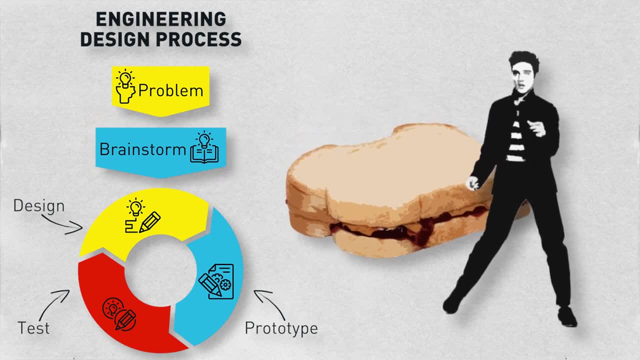 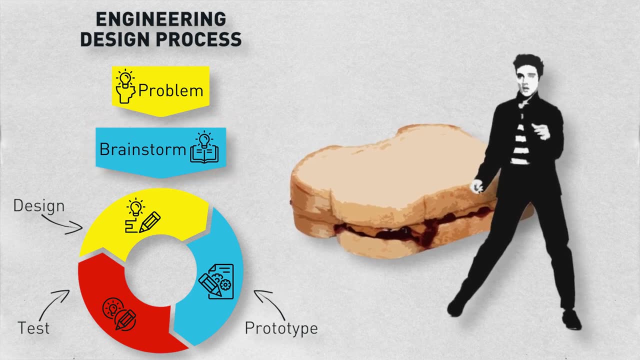 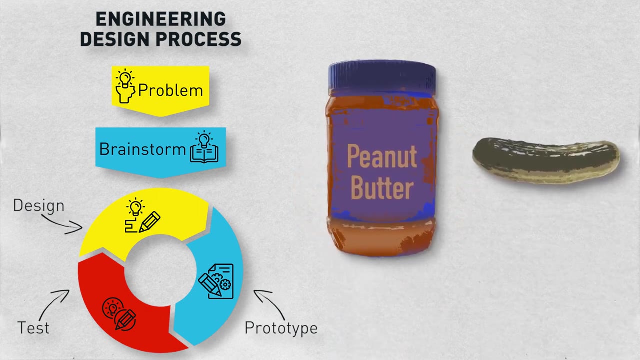 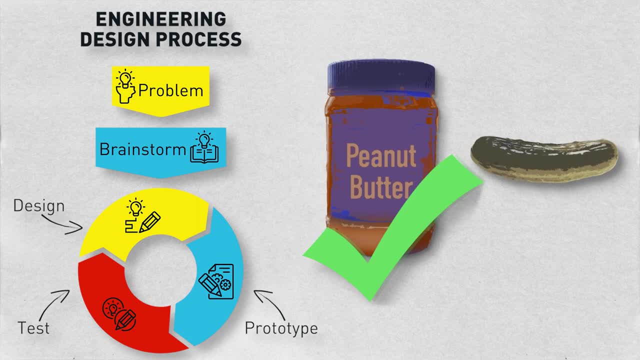 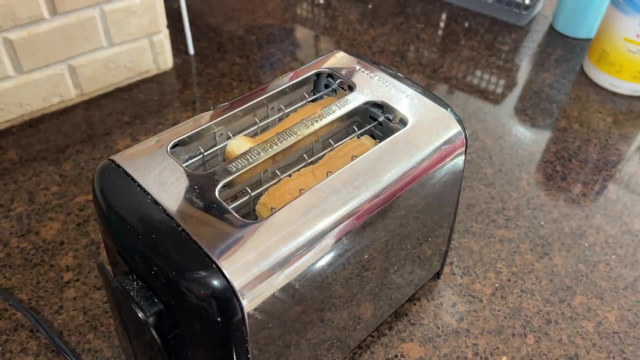 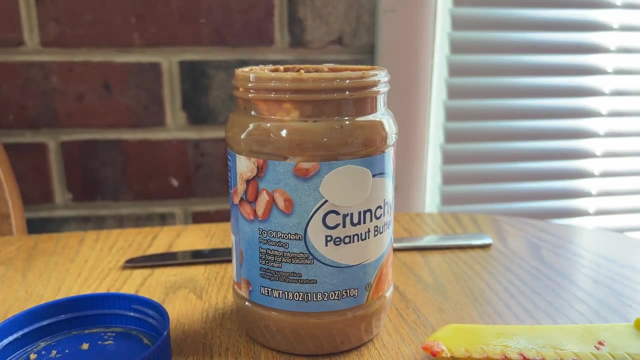 We look at several solutions and then choose the best one to test. I love the idea of using toasted bread to support my sandwich better. Maybe some cut up strawberries for texture? What if we tried chunky peanut butter? Yep, that's it. 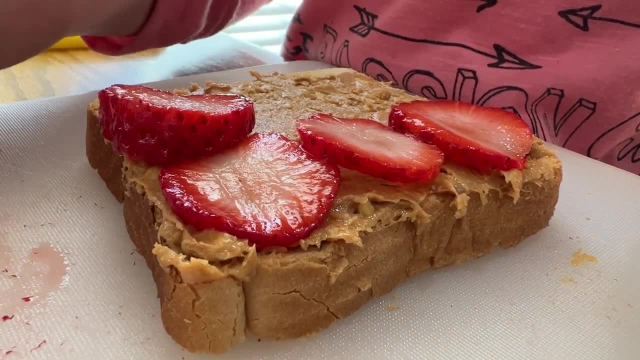 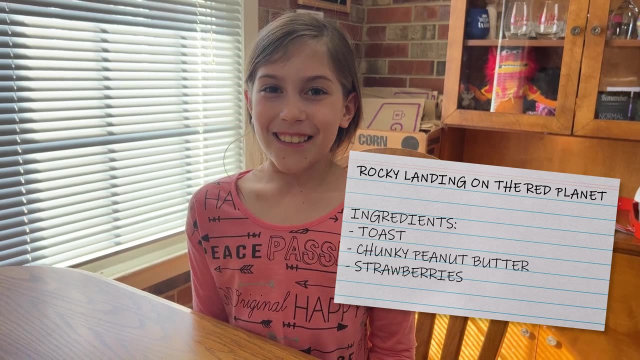 I'll make a peanut butter sandwich on toasted bread with strawberries and chunky peanut butter. I'll call it the rocky landing on the red ground. I'll call it the rocky landing on the red ground. I'll call it the rocky landing on the red ground. 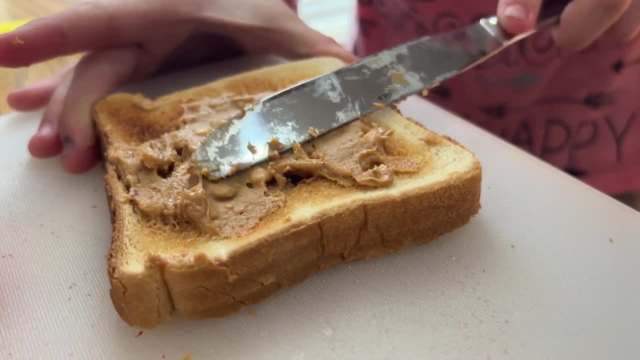 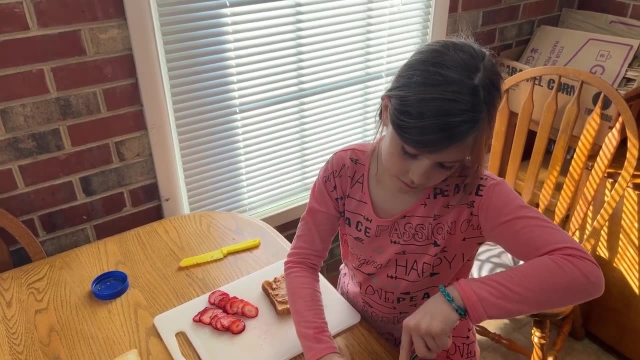 Time to prototype. That means we get to build a model and test how it works- Or, in this case, it's time to make our sandwich. You can also think about the prototype stage like writing a rough draft of a story. You can also think about the prototype stage like writing a rough draft of a story.